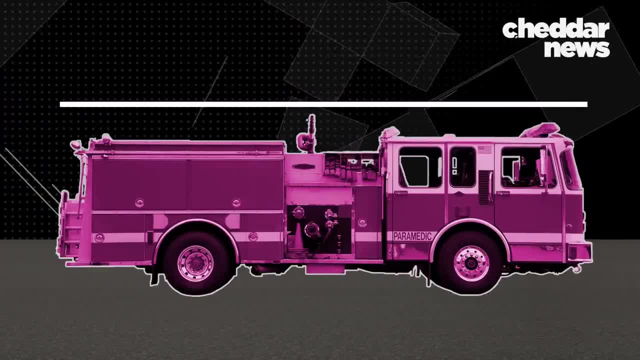 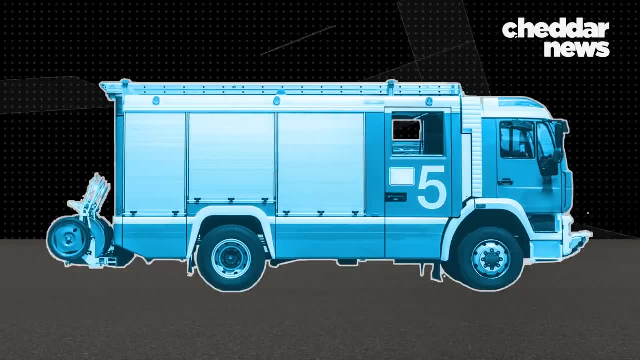 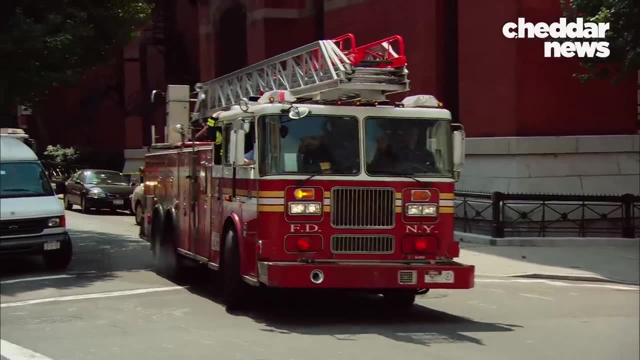 The average American firetruck spans 40 feet, is 10 feet wide and 12 feet tall, and their international competitors are usually much, much more compact, Not to mention the US. one just looks old. It's a difference that's resulted in contrasting approaches to firefighting. 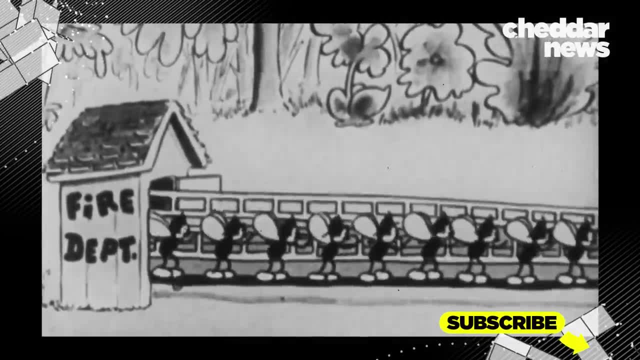 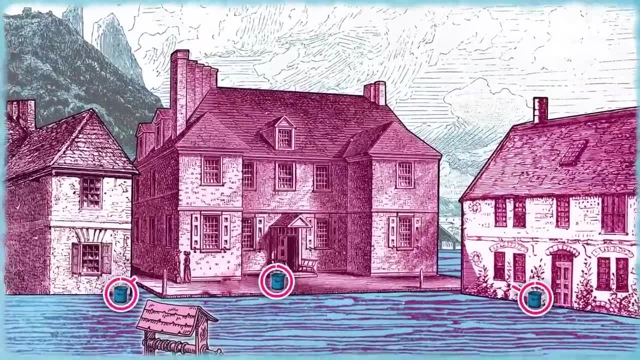 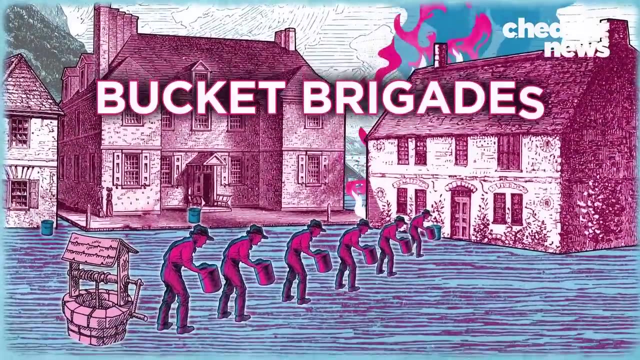 Bigger might not always be better. American firetrucks weren't always this massive. During colonial times, most homeowners kept buckets on their front porch, And when members of the Rattle Watch would raise the alarm, citizens would form bucket brigades and pass the buckets from the water source to the fire. 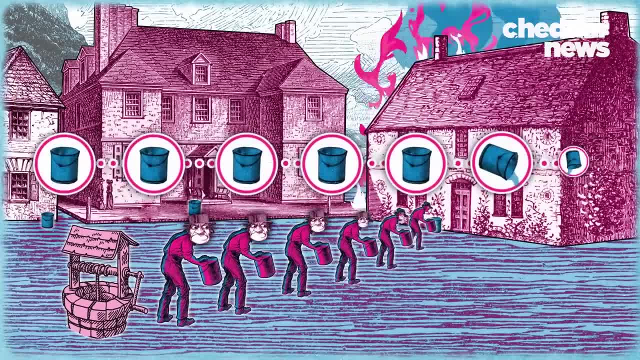 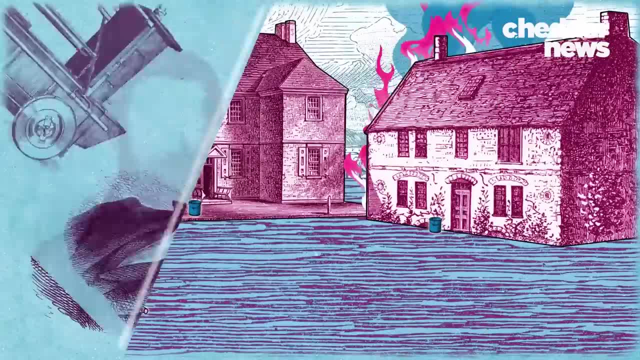 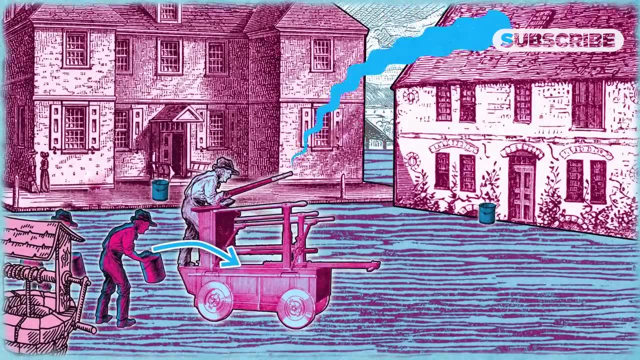 Now, this obviously required a lot of cooperation and clearly wasn't that efficient. So in 1721, Richard Newsham patented a type of fire pump. The pump was mobile, mounted on a wooden chassis, But bucket brigades would still have to dump water into the hopper. 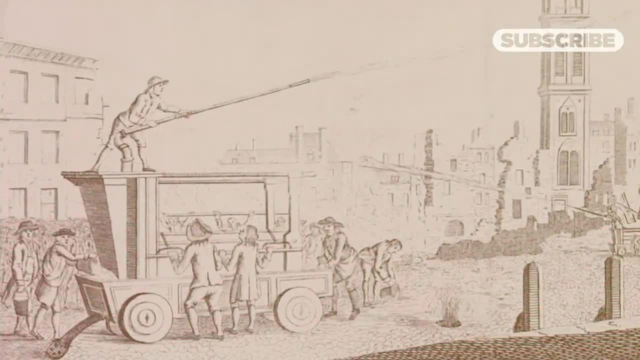 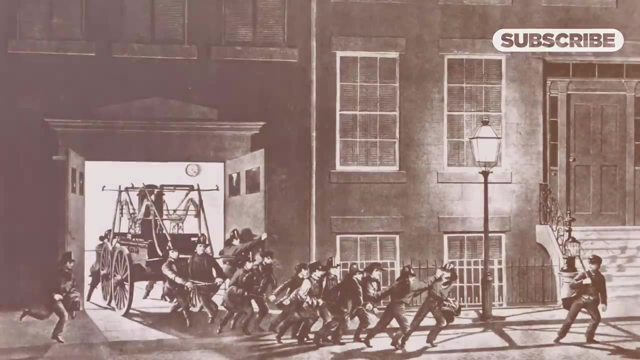 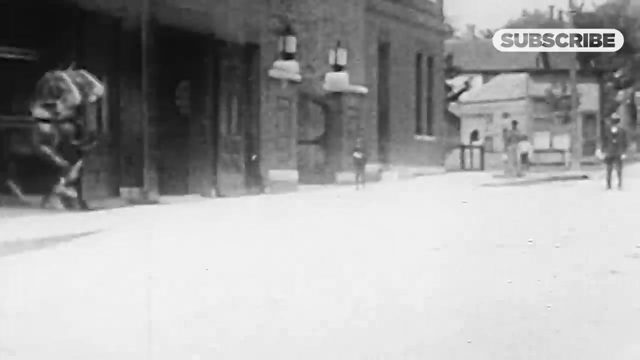 So, as you can imagine, these weren't the most effective either. Firefighters would show up late to a scene, often exhausted from lugging around all the equipment. In many cases, fires died out before the brigade even arrived. By the turn of the 19th century, larger US cities relied on horse-drawn wagons with 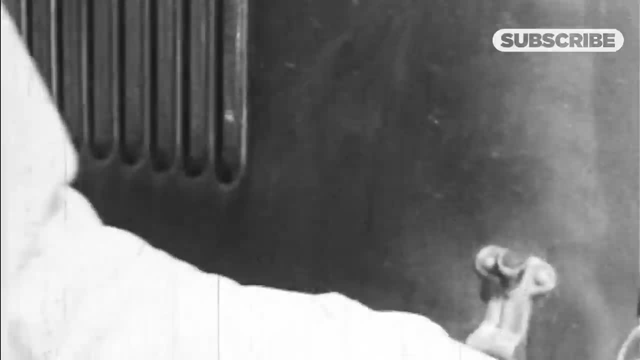 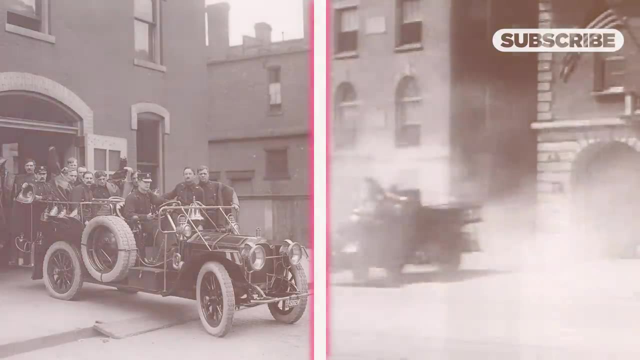 steam-powered wagons. Finally, the internal combustion engine allowed for the introduction of the fire truck, which hit the roads in the early 1900s. Throughout the first half of the 20th century, American cities began growing taller and taller. 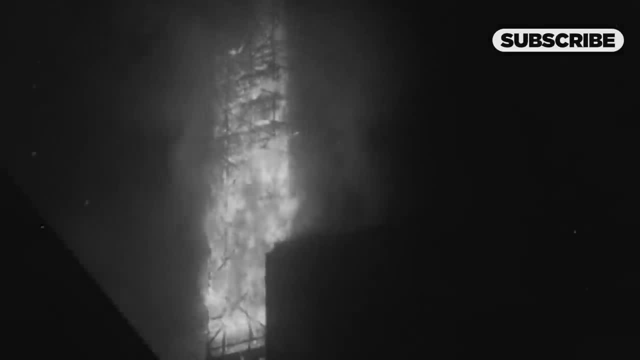 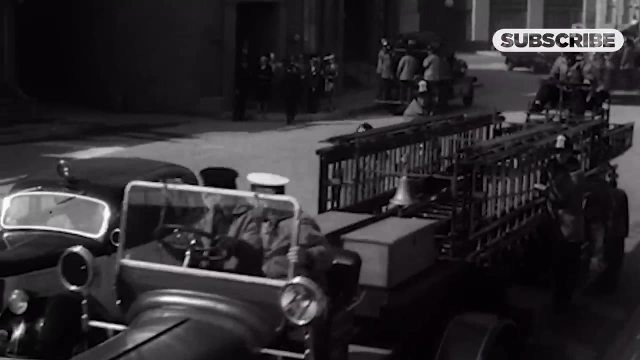 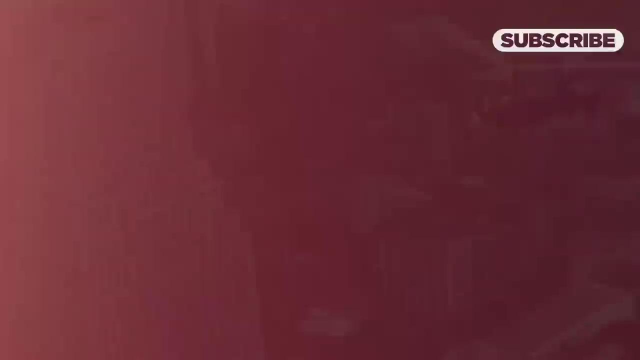 And this presented a new kind of challenge. So New York firefighter Daniel Hayes designed the Hayes Ladder, which was mounted directly on the fire truck and could be raised and lowered. In the years following World War II, fire departments added these so-called cherry pickers to their trucks. 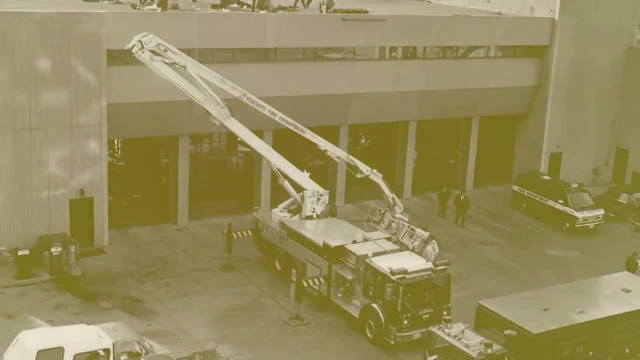 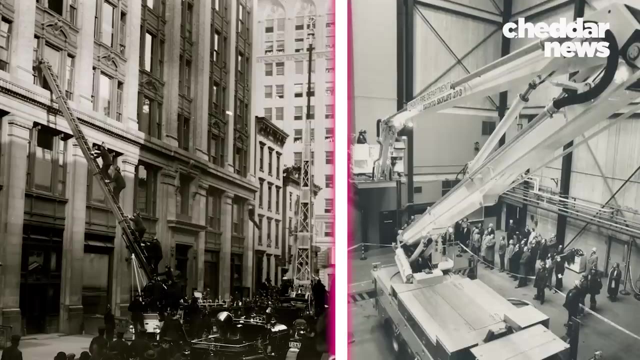 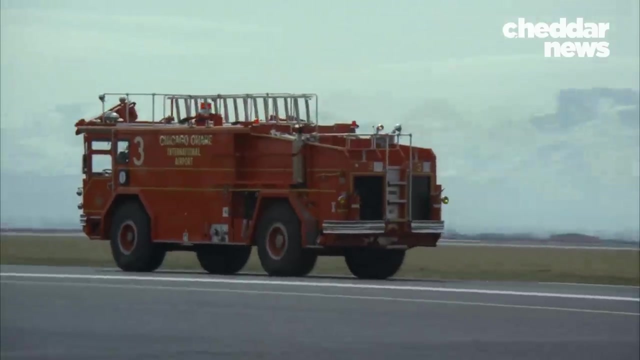 This bucket, attached to a bending arm, allowed firefighters to position themselves closer to previously unreachable corners of buildings. Both ladders and the cherry pickers required a larger, sturdier chassis. From then on, the fire truck continued to grow larger, as each new model was designed to house more equipment. 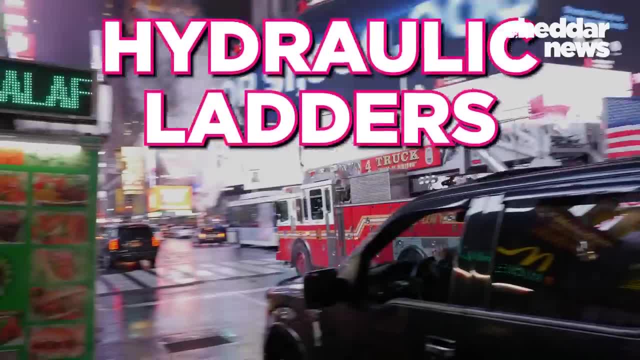 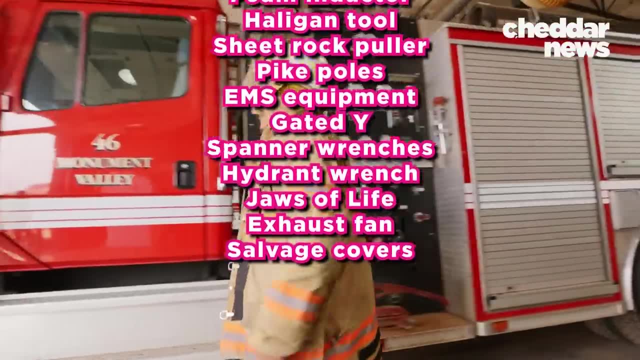 Today, the average truck is loaded with pumps, Hydraulic pumps, Hydraulic ladders, Tanks that can hold roughly 400 to 500 gallons of water And a slew of other equipment. Also, the term fire truck has come to encompass a variety of search and rescue vehicles like 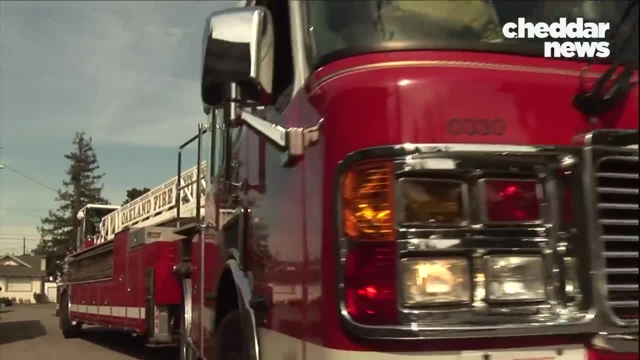 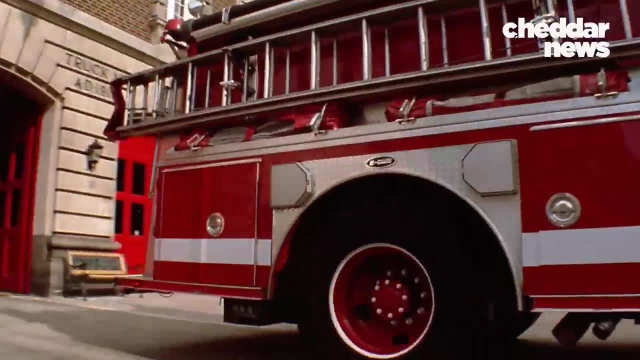 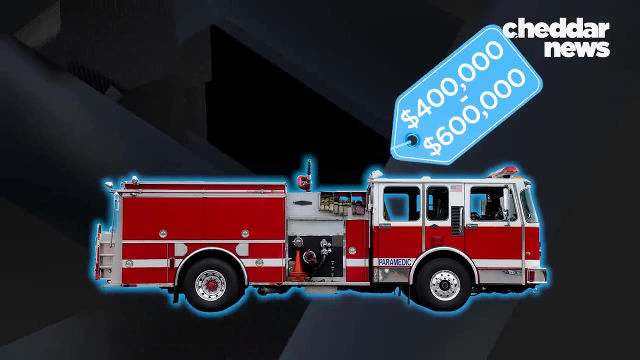 ladder trucks, engines and tiller trucks. But regardless of the specification, almost all American fire trucks are larger And that comes with a larger price. The average cost of a widely used Type 1 engine goes anywhere from $400,000 to $600,000, and a 100-foot aerial ladder alone goes for around $1,000,000. 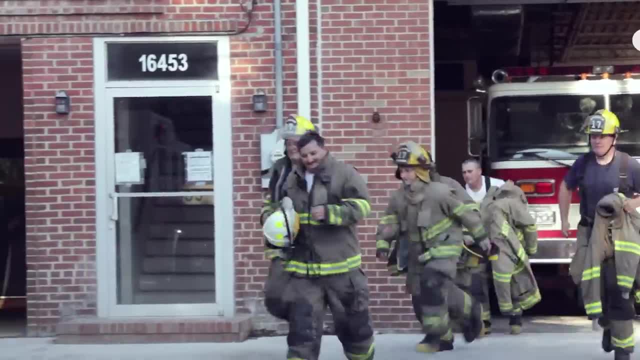 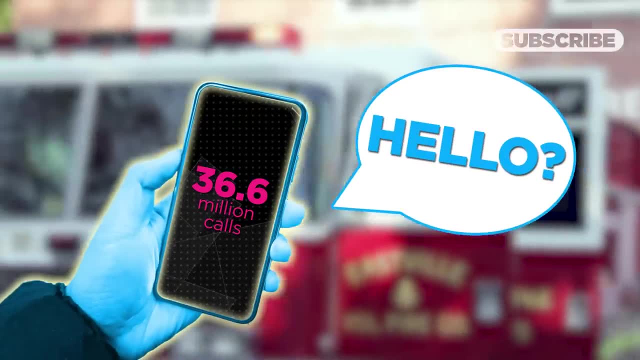 That's a big price tag when few of the calls forwarded to fire departments are actually fire-related. Of the 36.6 million calls made to all of the US fire departments in 2021, only 1.3 million, or about 4%, were fire-related. 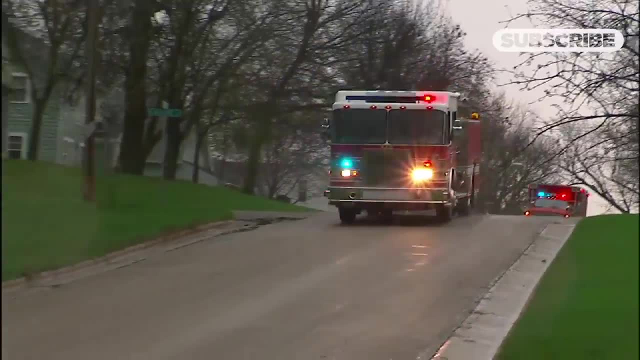 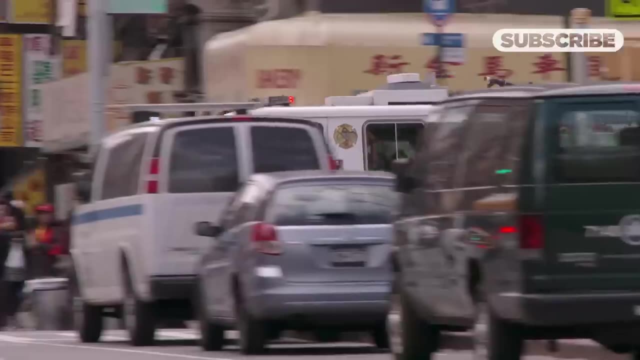 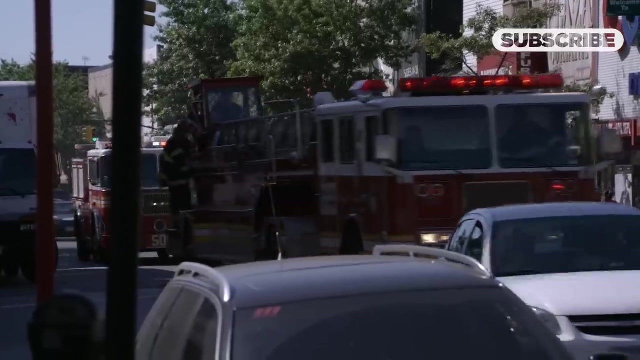 A large majority of the other calls are to accompany ambulances to the scene of auto accidents and other fires. In addition to the price tag, heavy-duty vehicles like fire trucks can pose risks to smaller cars, pedestrians and cyclists. They're heavier and have a longer braking distance. 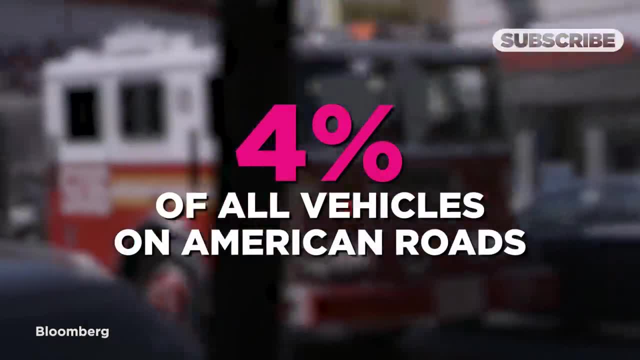 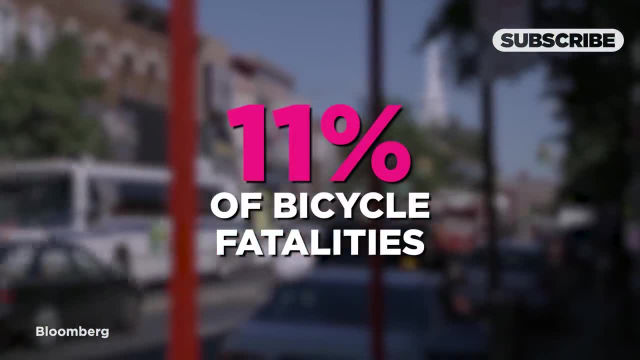 Heavy-duty trucks make up just 4% of all vehicles on American roads, Yet they account for 7% of pedestrian fatalities and 11% of bicycle fatalities. In the summer of 2018, lawmakers in Baltimore pushed for the addition of fire trucks to 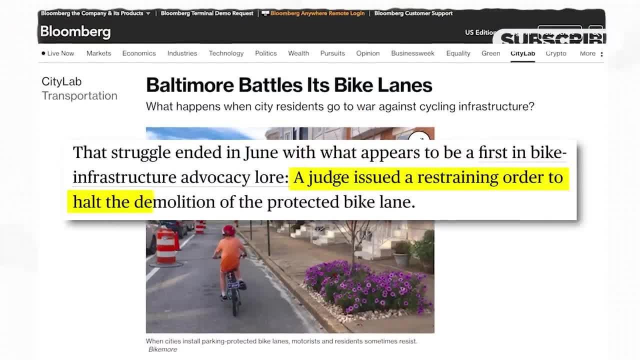 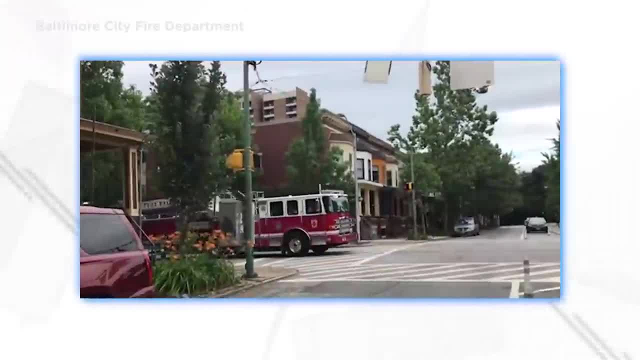 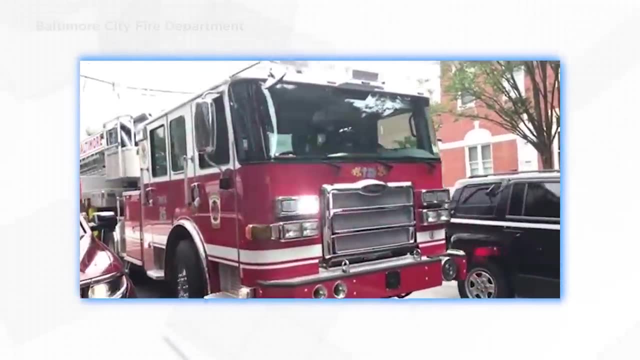 the scene, which would in turn create narrower street lanes for cars, But the Baltimore fire department opposed the proposal, releasing a 9-minute video suggesting bike lanes would impede their ability to maneuver to a scene. The 10-foot-wide American fire truck struggles to squeeze through traffic on the average. 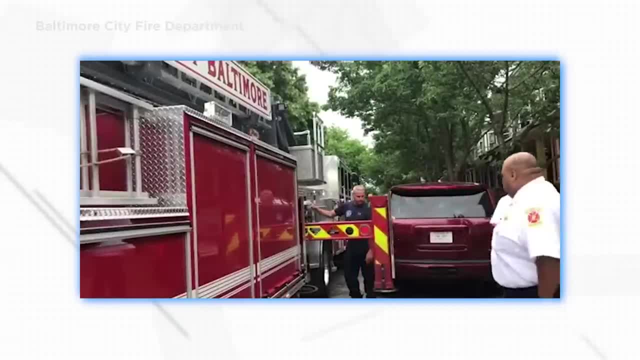 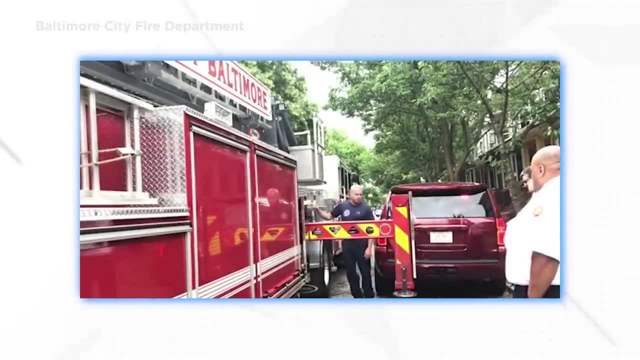 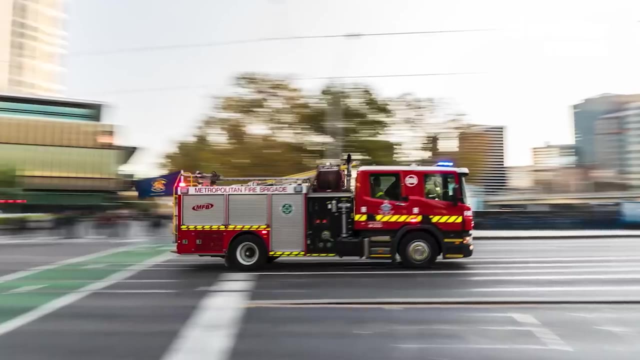 10- to 12-foot-wide American road lanes, especially in older cities with thinner, more congested streets. So what should a fire truck do? Well, maybe like this: In Europe, streets tend to be tighter, so fire trucks are shorter, narrower and more. 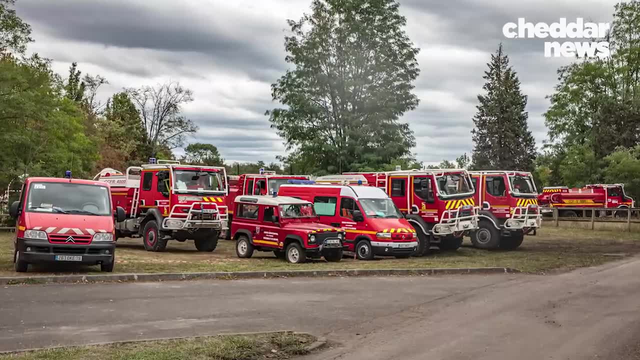 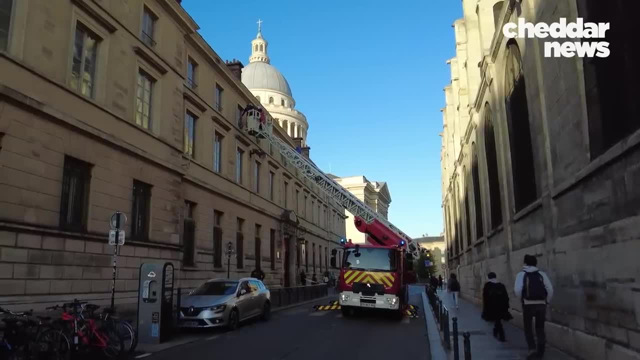 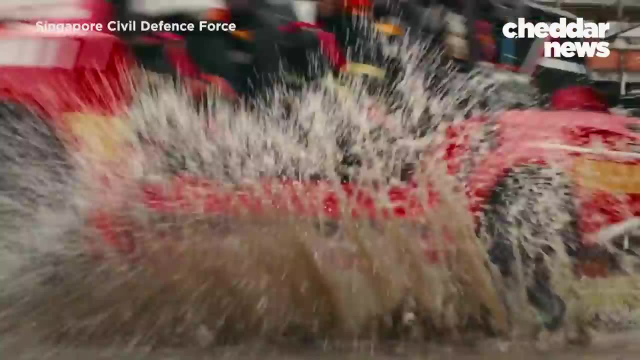 compact, making them far more maneuverable. Their aerial ladder, fire trucks, can also reach just as high as the American counterpart, even though they're a third shorter. In Singapore, fire trucks, or so-called red rhinos, are even more compact, yet they still